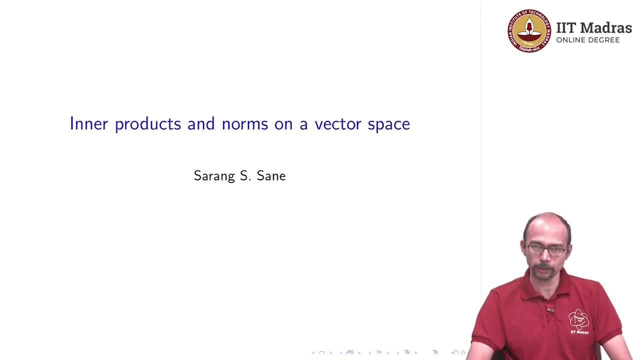 So we will see that the notion of an inner product generalizes what is a dot product, and the notion of a norm generalizes what is the length. So the point here is that we can do this for any vector space. So let us start by the. 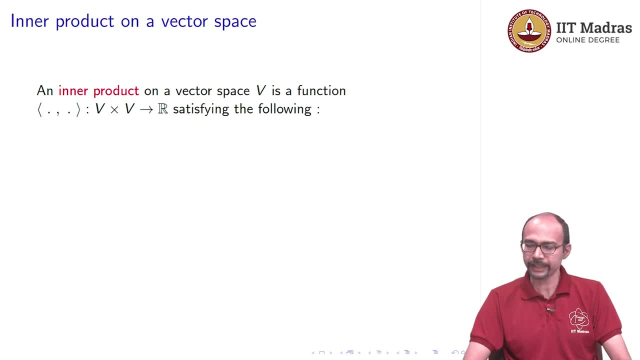 by defining what is an inner product. So an inner product on a vector space, V is a function, which is which takes two vectors as input. So that is why the dot, comma dot. So in place of the dots you will have vectors. So it is a function from V cross V to R. So 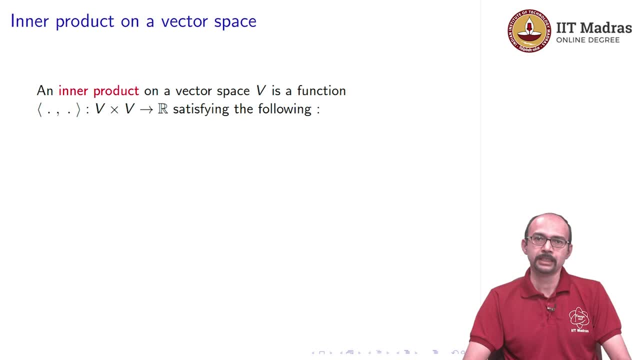 it gives, it produces a real number For each pair of vectors. it produces a real number And it satisfies the following. So if you take into, if you apply this to V comma, V, that means you take just one vector and you think of it as: 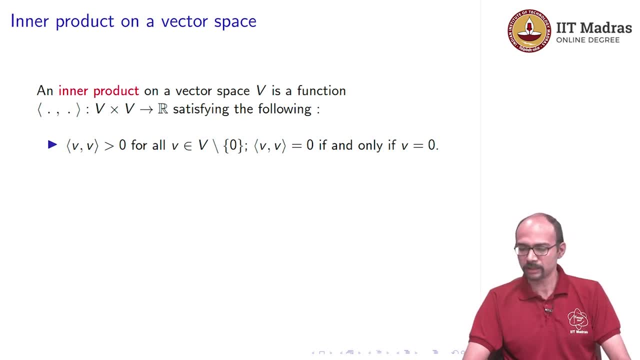 as the tuple V comma V, then the inner product of V with itself. that is how we describe, we will say V comma V. this angle brackets. this must be positive- strictly greater than 0, if V is non-zero, and it will be 0 precisely when V is equal to 0. 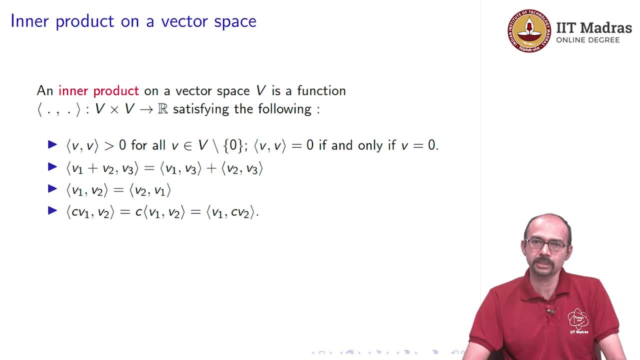 And then you have these three things which are which I have put together because they are called these three things. this is saying that it is bilinear. So these three things say it is bilinear. So V1 plus V2 is comma, V3 is V1 comma. V3 plus V2 comma, V3, and V1 comma V2 is V2 comma V1. 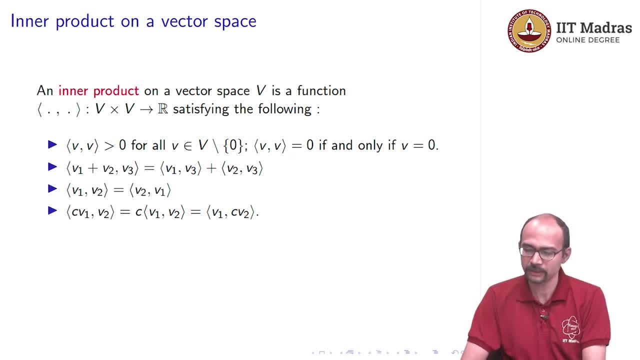 And C times V1 comma. V2 is C times V1 comma V2, which because of your previous thing can be written also as v1 comma c times v2, where c here is a real number, it is a scalar, So I will. 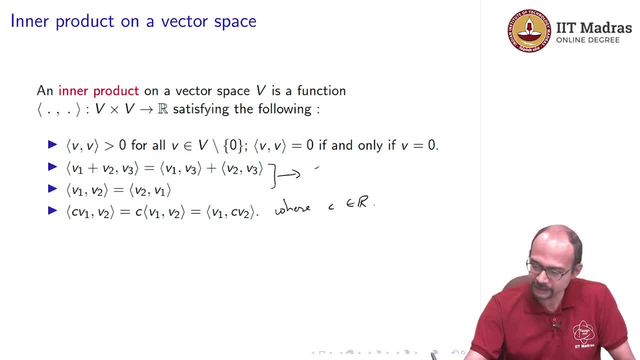 also point out that using these two we can get that v1 comma v2 plus v3 is equal to v1 comma v2 plus v1 comma v3, because v1 comma v2 plus v3 is v2 plus v3 comma v1,, which is: 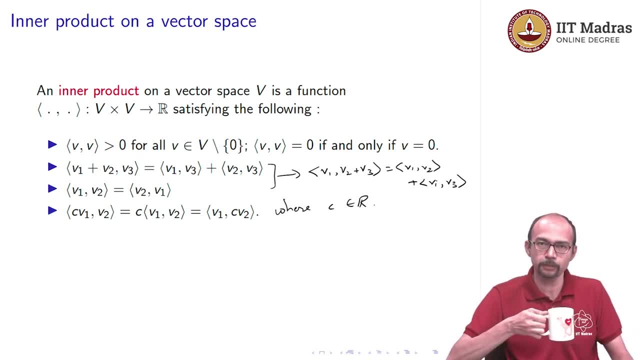 then v2 comma v1 plus v3 comma v1, and then you can flip those again to the other side. So now these three together are what is called bilinear. So this is a bilinear map, The first one, The second one. 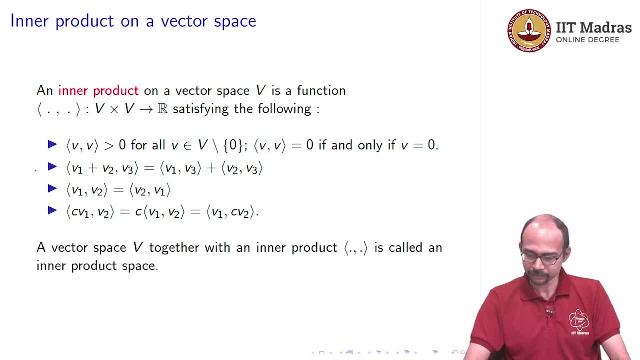 and third. So a vector space together with an inner product is called an inner product space. So I will underline this is called an inner product space. this is a definition And maybe I will just put in the conclusions we drew. So the conclusions we drew, 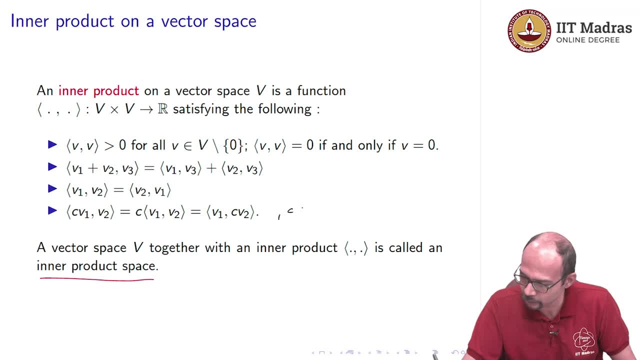 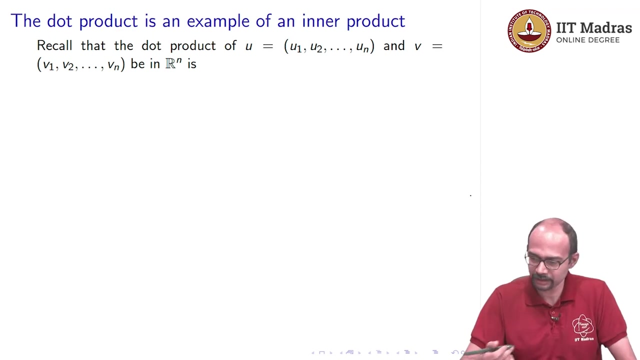 before. where that? so first of all here, this is not a conclusion, this is a hypothesis. C is a scalar and the conclusion out of this was that v1 comma v2 plus v3 is v1 comma v2 plus v1 comma v3.. So the dot product is an example of an inner product. this is what I started with. 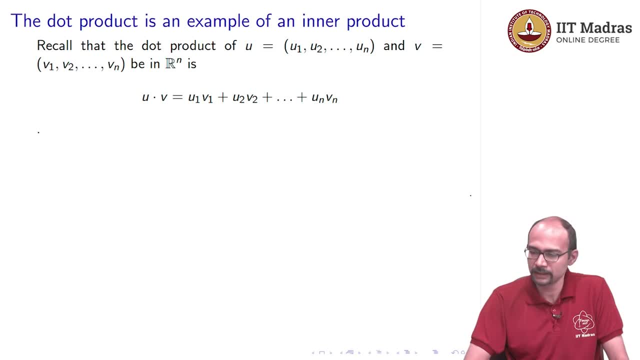 So recall that the dot product of u and v in Rn is u, dot v is u1, v1 plus u2, v2 plus u and vn. I apologize for this ugly look in full stop, which should have been here. And this yields a function. 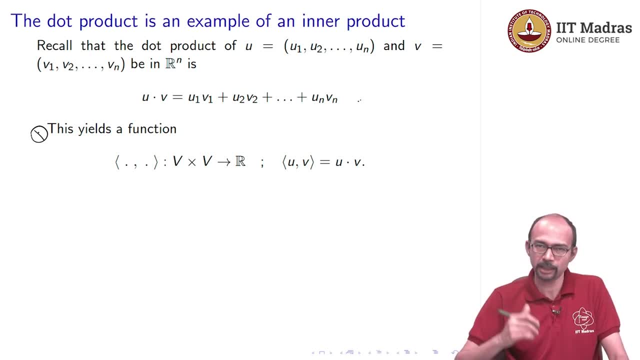 which is given by u comma v is u dot v. angle brackets: u comma v is u dot v. So why is this inner product? So we have to verify the three axioms, the four axioms we had. So we know already that if u comma u is so, this is u1 squared plus u2 squared plus u n squared. 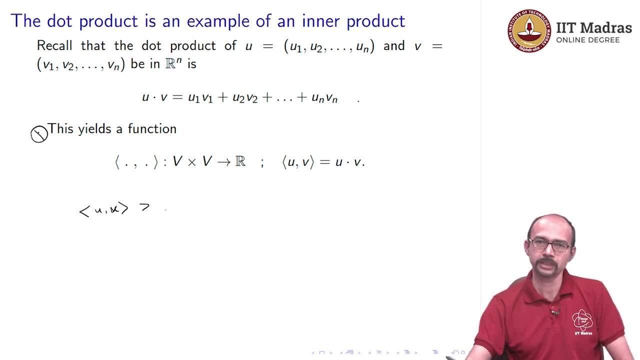 for real numbers, squares must be positive. sum of squares is positive. So that means this is greater than 0 if u is not 0. And this is equal to 0 exactly when each ui is 0. So ui is 0 for all i. 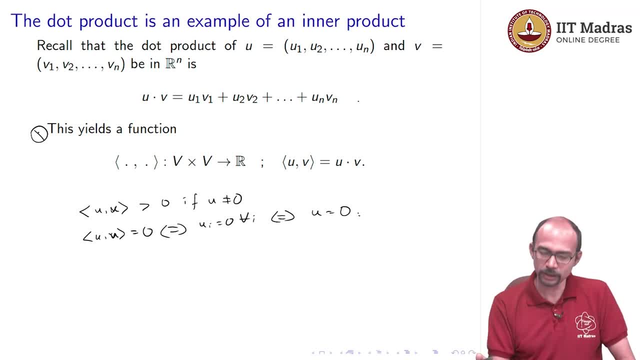 which happens precisely when u is 0.. So we have proved the first one, And the other three just follow from the form of this equation. So if you have u plus u prime dot v, you can check that this is actually u dot v plus u prime dot v. 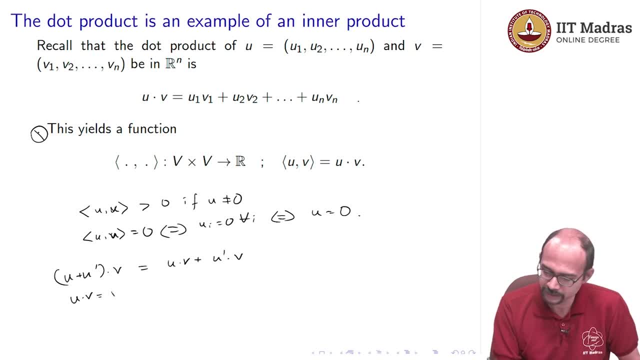 And similarly, if you have u dot v, this is the same as v dot u. that is clear from the equation because real numbers you can they commute under multiplication. And then clearly, if you have cu, which is u dot v, this is c times u dot v, because c multiplies into each component. 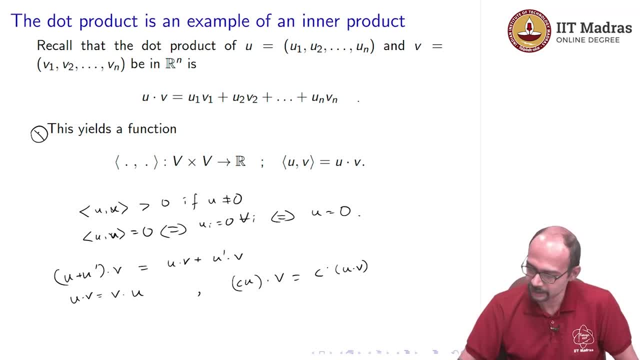 So for each component you will have it over there and then you can take it out. So this completes the proof that this is indeed a inner product. So the dot product is an inner product. So let us now look at an example of an inner product on R2,. 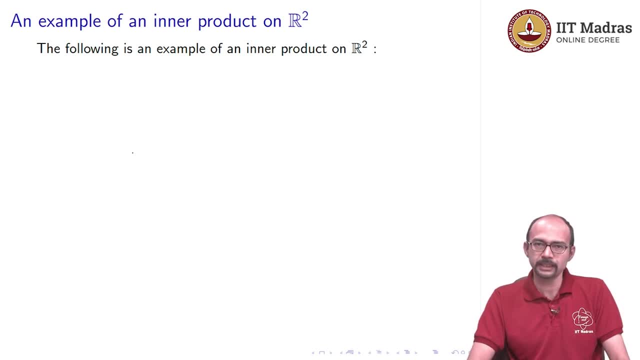 which is this is a. this is not the standard inner product that we saw, the dot product that we saw earlier. this is a slightly different example. So here is the definition: u comma v is x1, y1 minus x1, y2 minus x2, y1 plus 2 times x2 y2.. So where u is x1, this is a typo here. 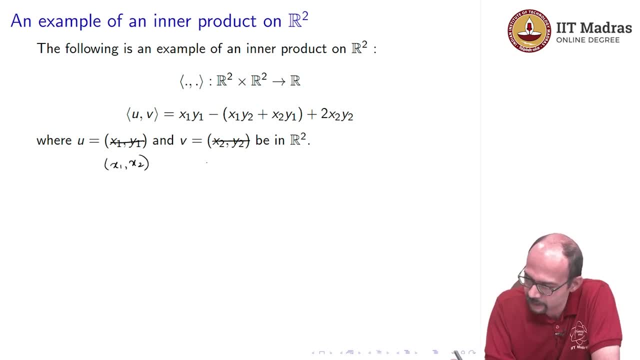 So u here is x1 comma x2, I think, and v is y1 comma y2.. So the standard inner product that we saw was so: if you do u dot v, u dot v is x1 y1 plus x2 y2.. So, in terms of, is x1 y1 plus x2 y2.. The inner product here is: 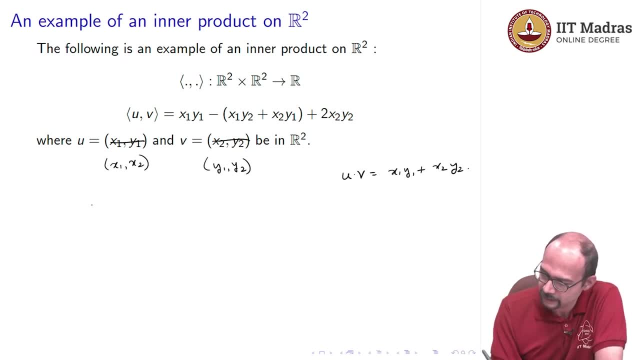 slightly different, as you can see. So why is this an inner product? How do I prove that? So this is proved by by looking at the following: If you look at this expression, you can write down the matrix for this expression. So you have x1, x2, and then you have y1, y2.. 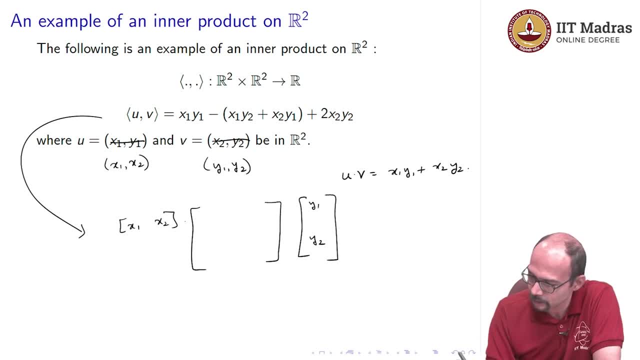 And then let us see: So you have x1- y1, the coefficient is 1, x1- y2, the coefficient is minus 1.. So I believe this will be minus 1 here, And then this is minus 1, and then this is 2.. 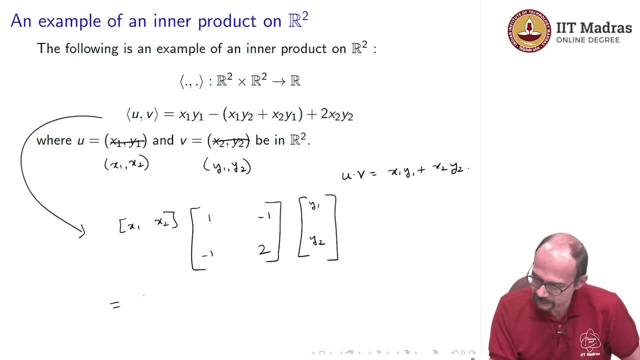 So if you multiply this, let us see what we get, you get exactly. So the first term is x1 minus x2, the second term is minus x1 plus 2 times x2, times y1- y2.. And if you work out what this is, this is x1 y1 minus x2 y1. 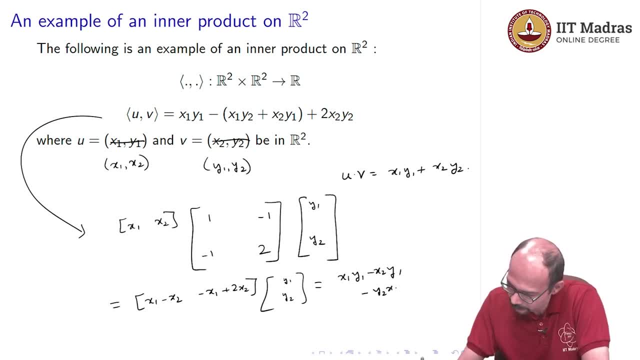 So this is minus y2 x1, plus 2 times x2- y2.. So this is exactly what we have up here. This expression and this expression are the same. So this is a different expression from the inner product, which is x1 y1 plus x2 y2.. And now how do? 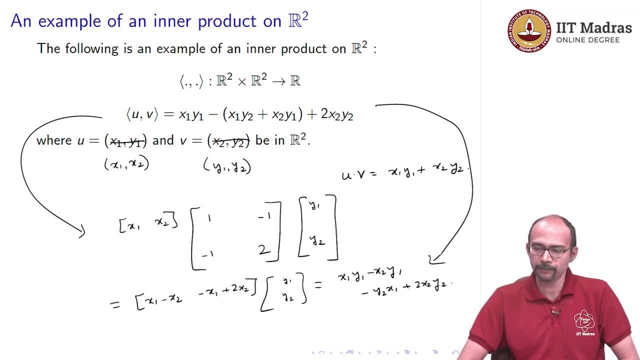 I use this matrix form to conclude that it is an inner product. So the reason: so I can use the matrix form to conclude that it is an inner product because the bilinearity part follows directly And the symmetry part follows, because this is a symmetric matrix. So if I want to do 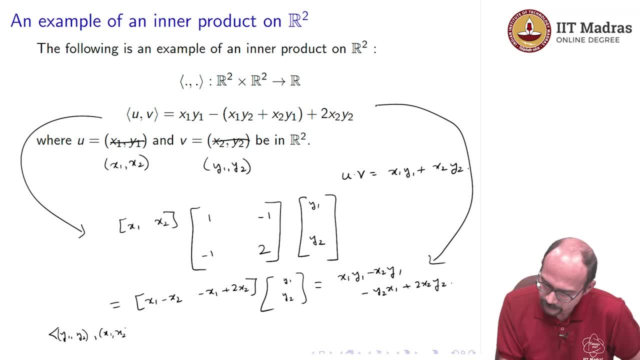 y1, y2, comma, x1, x2, then you can see that this is exactly writing y1, y2 here, writing the same matrix here and x1, x2.. But this is a real number, So I can. so this is the same. 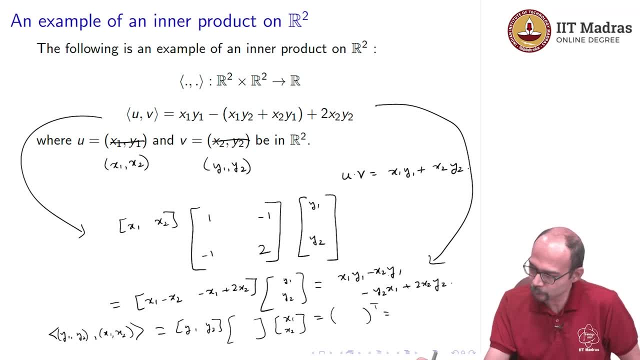 as it is transpose. this is the same thing: transpose. And if you do the transpose, you will get this, because the matrix in the middle is a symmetric matrix, So it is transpose is itself, So that is why it is symmetric. that is the second property. 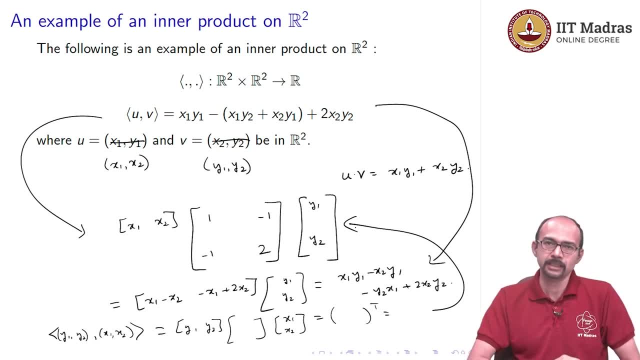 And then bilinearity is because matrix multiplication respects addition. So if you have, so it distributes over addition. So if you have x1, x2, let us say plus x1, prime, x2, prime, then over here you will, you will, that will distribute. 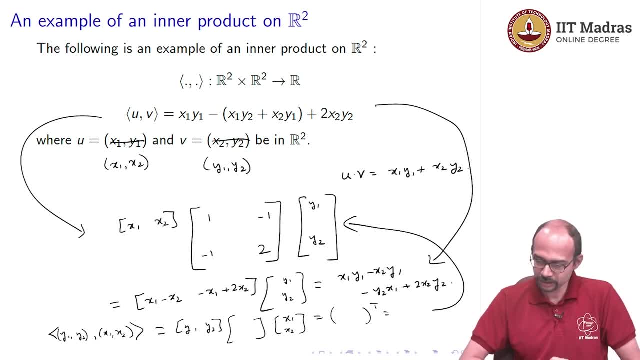 and it will give you what you want. That is the first thing. And then c times x1, x2, again, because constants come out of matrix multiplication. it will follow from there. So I will urge you to check that fact, because these two expressions are the same So. 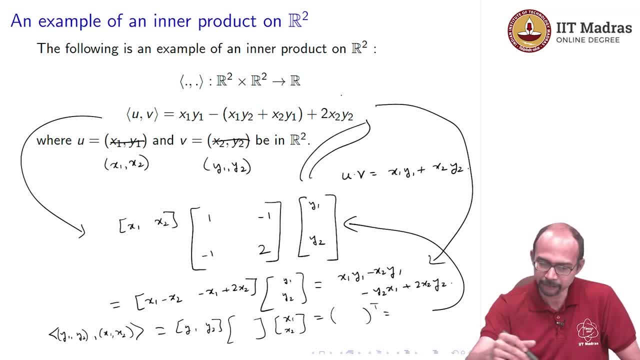 the key point here is: these two expressions here are the same, So maybe I will draw that better. These two expressions are the same, So you can check it from there. So the only remaining thing is that this is always positive. So if you put x1- x2 in place of y1- y2, what do you get? 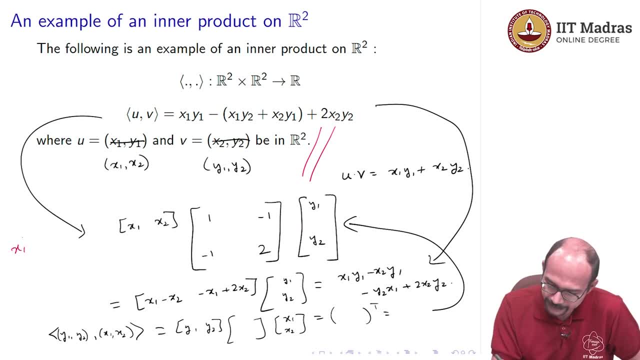 So you get x1 squared minus x1, x2 minus, or rather plus x1 x2, that is 2 times x1, x2 plus 2 times x2 squared. So this is x1 squared minus 2 times x1 x2, plus 2 times x2 squared, And you can write this as x1 minus x2 squared plus x2 squared. 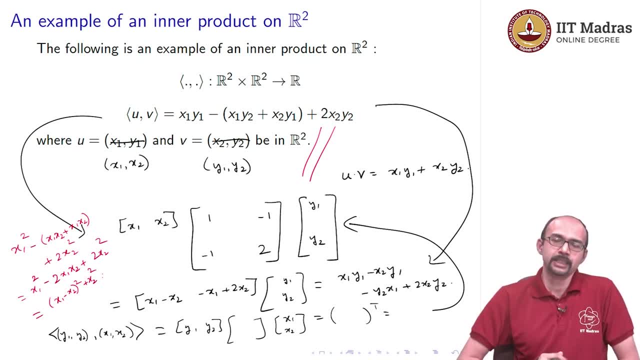 So this is the sum of squares. Again, it must be positive. If it is equal to 0, then both the terms which are squares are 0. That means x1 minus x2 is 0 and x2 is 0. Once x2 is 0, x1 must be 0.. 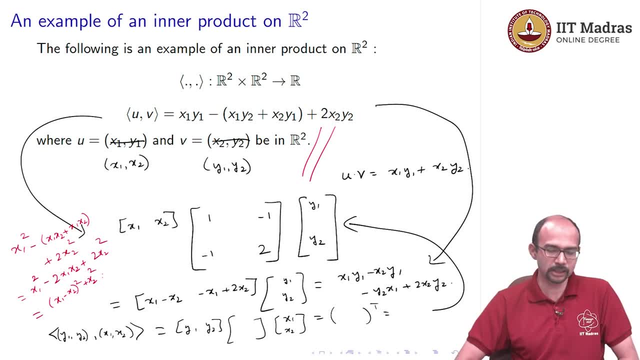 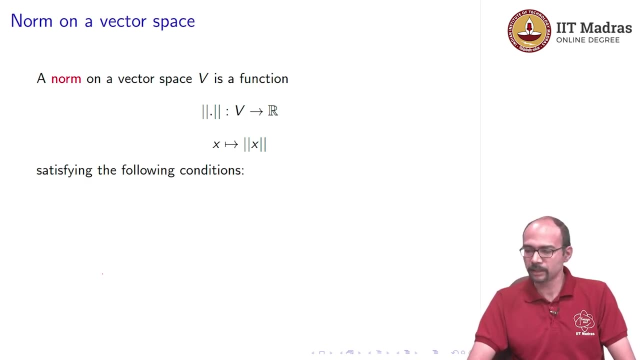 So both x1 and x2 are 0. So that tells us that it is 0 exactly when u is 0. So this proves that it is an inner product on R2.. Let us define what is a norm. So norm on a vector space is a function. It is indicated by that. 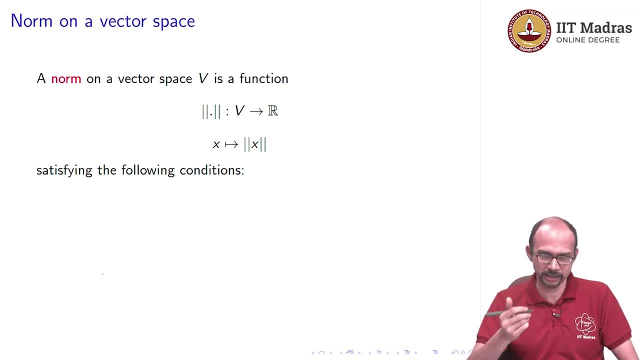 double lines And we have seen these double lines in the previous, in the previous video. x goes to norm x, y the following conditions: So norm of x plus y is less than or equal to the norm of x plus norm of y. Norm of c times x is absolute value of c times norm of x. So remember in the previous 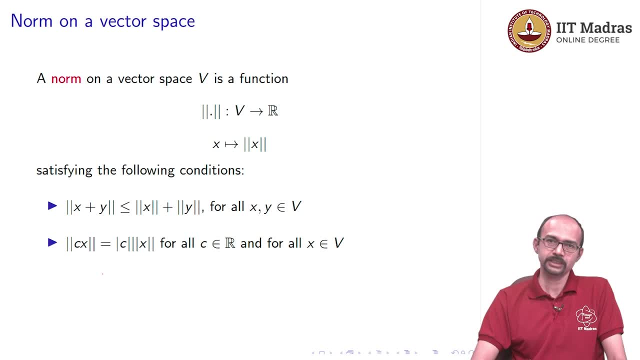 video. this norm was supposed to represent length, So since it represents length, it better be positive. And so, if you have, if you scale it, the length better remain positive. That is what is being reflected here. So positive. that is what is being reflected here. So positive, that is. 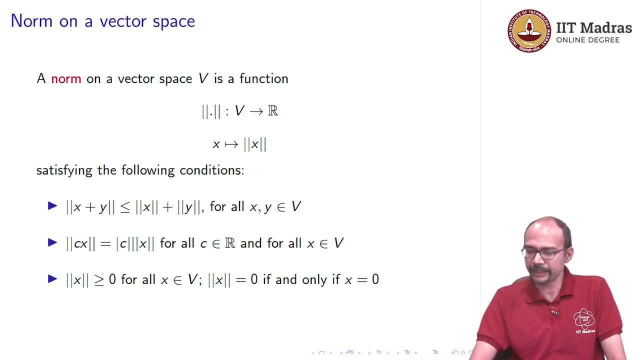 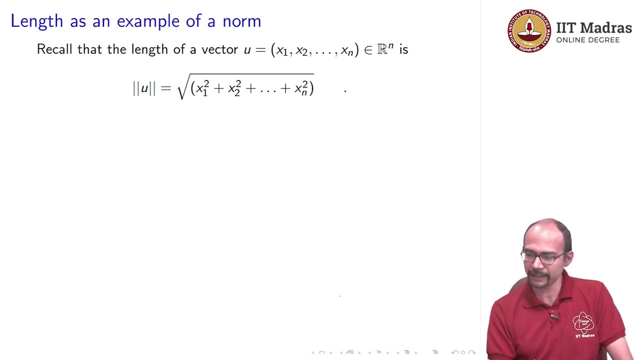 positivity is coming in. the third axiom Norm of x is always greater than 0, and it is 0 precisely when we are dealing with the 0 vector, if, and only if, the vector x is 0. So let us recall the length of a vector. This is the comment I made in the previous slide. 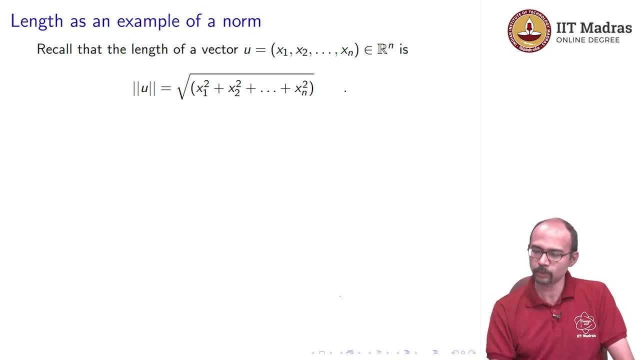 u. it is given by this expression root of x1 squared plus x2 squared plus xn squared, And this is actually a norm. So we have to say that the three previous conditions are satisfied. As I said, if you multiply this by c, this is clearly root of c squared, x1 squared plus c. 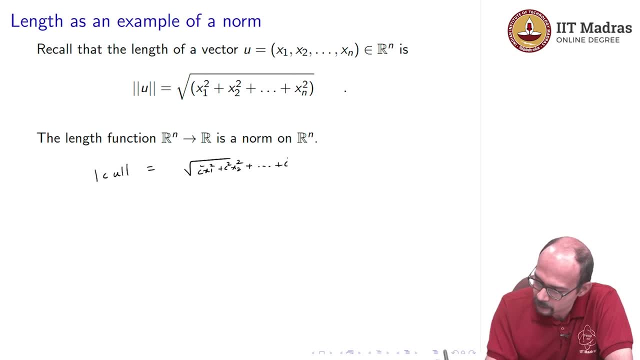 squared, x2 squared plus c squared, xn squared, And the c comes out, but with an absolute value, And the remaining part is norm of u. length of u. This should have been two parts. Let us see when this is 0.. This is 0.. We have actually checked this, So the length is 0. 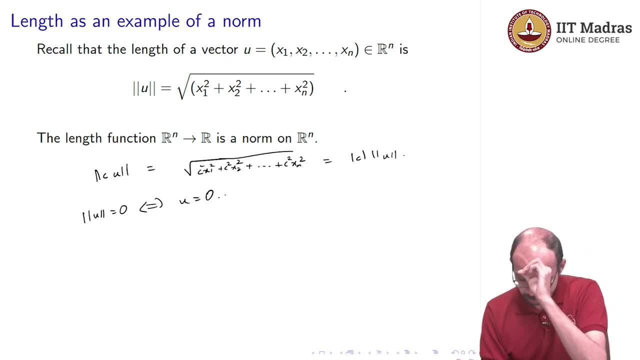 exactly when u is 0.. This is something we know, which leaves us with the triangle inequality, Namely, if you take two vectors, u plus v, then you compute the sum. So this is root of x1 plus y1 squared plus x2 plus y2 squared plus xn plus yn squared. 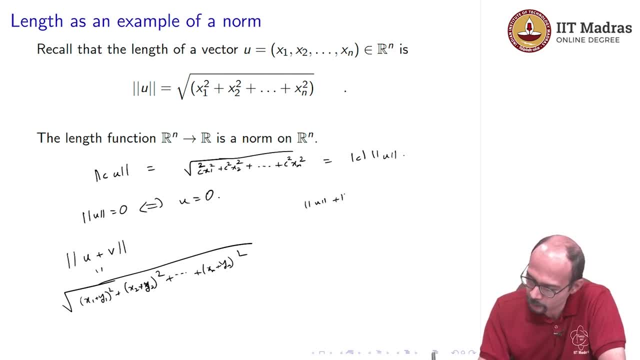 And on the other hand, we have norm of u plus norm of v, which is root x1 squared up to xn squared. This is root y1 squared plus all the way up to yn squared. So I want to say that these, this sum is: 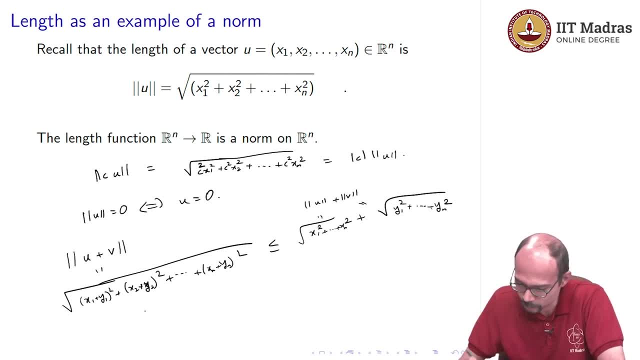 greater than greater than equal to y1 squared and greater than equal to yn squared. So I want to say that these this sum is less than or equal to that sum, and this is something that we know is true, and I will: yn squared. This side, you get x1 squared plus all the way up to xn squared plus y1 squared. 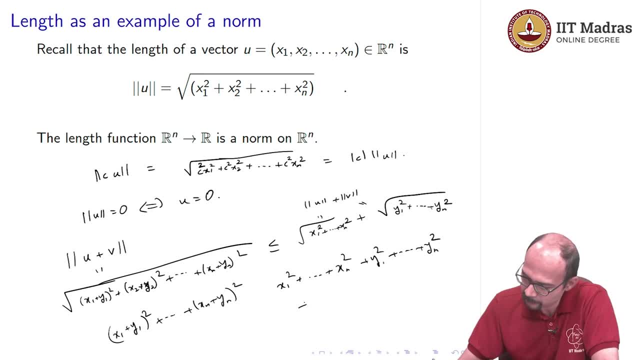 all the way up to yn squared, and then plus 2 times this root, and then y1 squared plus all the way up to yn squared, And then. so to compare these. so I want to compare these. so to compare these, you can expand the brackets. if you expand the brackets, 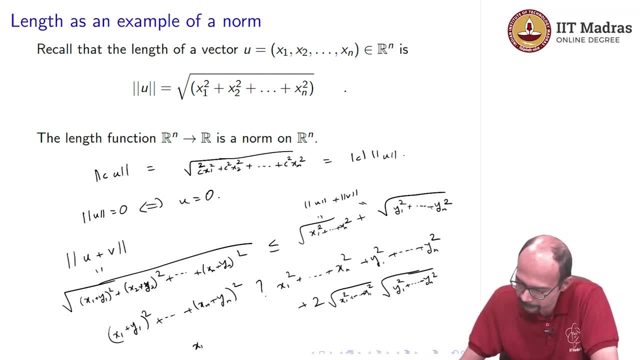 and you cancel off these square terms, you are going to have to compare 2 times x1- y1 plus 2 times x2- y2 plus 2 times xn- yn with this side. And now I will leave it at this point to: 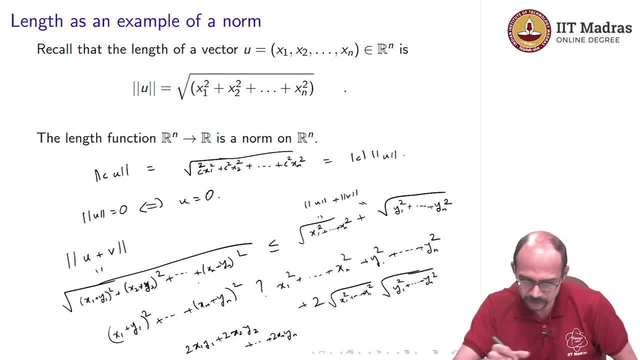 so you can cancel off the 2s as well. so you can. you have to compare this term with this term here And I will maybe not get into a proof that this is actually. this is less than or equal. it is a very something you can do. 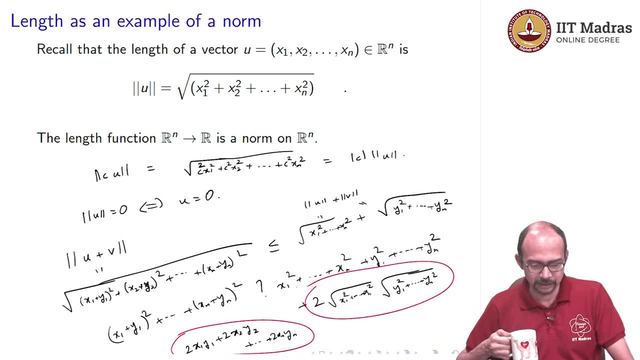 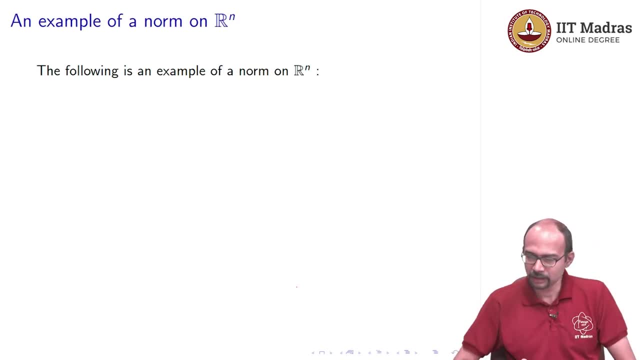 So the length function is a norm on Rn. So let us look at a norm on Rn. It is different from the length function. Namely, you can take the absolute values of the coordinates. So norm of u1, so this 1 is supposed to. I think this 1 has not come out the way I intended it to. 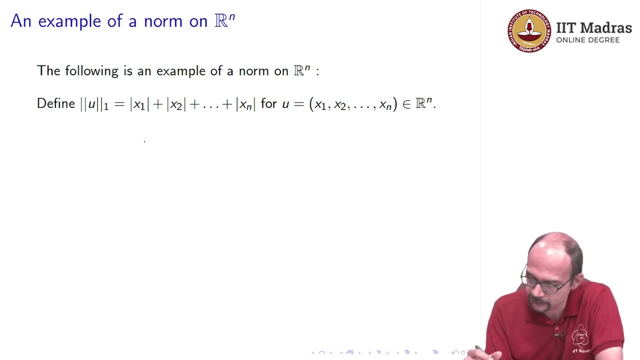 be. This should have been the subscript, but it has not come out as far as I wanted it Anyway. so define norm of u to be this: the absolute value of x1 plus absolute value of x2 plus absolute value of xn, then this is a norm. So let us check that this is a norm. 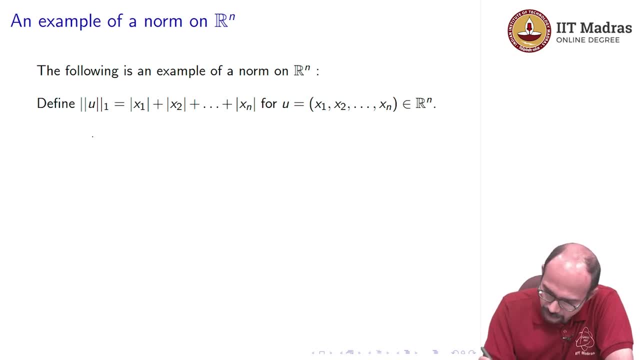 So, first of all, I want to check that if norm u1 is 0,- this is the third axiom- what happens? Well, this is a sum of non-negative integers, So this happens exactly when each xi is 0 in absolute. 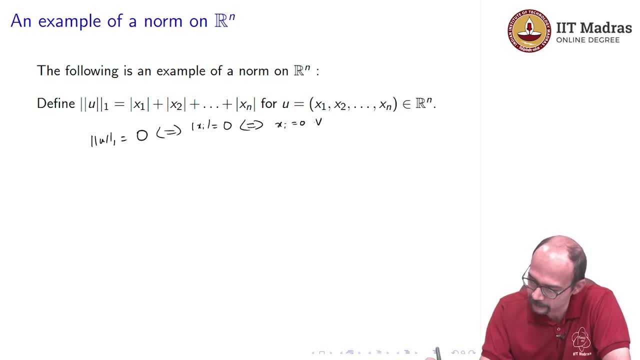 value, which is exactly happening when xi is 0 for all i, which is exactly saying that u is equal to 0.. So if this norm is 0, if this function is 0 on u, then u better be 0.. And, of course, 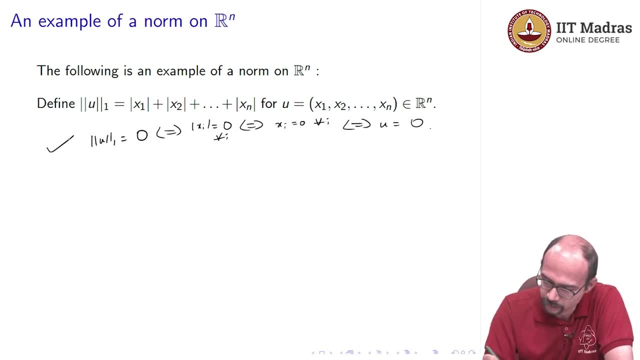 if u is 0,, then the function is 0. So this is one thing that we have checked. The other is: if you multiply this by a constant c, by a scalar, what happens? Well, each term is multiplied by c. 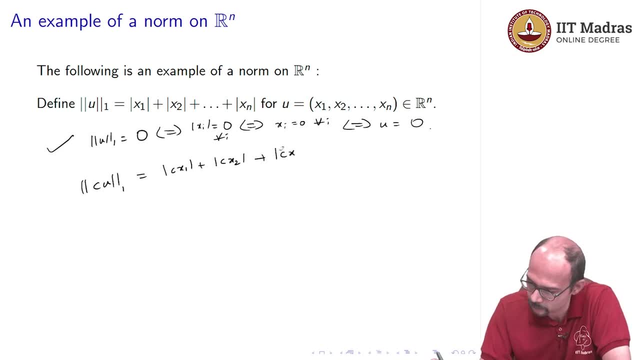 This expression- excuse me, I have to put in the dots. This expression and I can take my c out- common, because remember that the absolute value of two numbers multiplied is the absolute value of each multiplied. So you take c out. 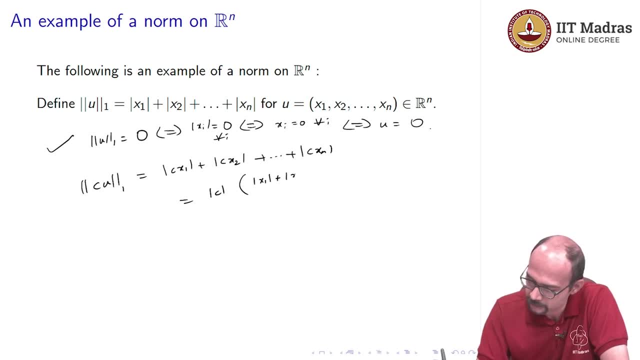 absolute value of c out common and you get x1 plus x2, all these in absolute value. So absolute value of x1, the absolute value of x2 all the way up to n, which is exactly what is the definition of the. 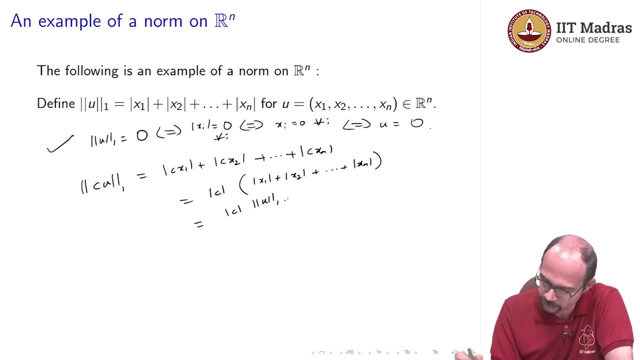 norm here. So c times this function. So this gives you one more thing. And then the last one that we have to do is the triangle inequality, which is saying that if you have u plus v, you take this. Well, let us write that down. That is x1 plus y1 plus x2 plus y2. 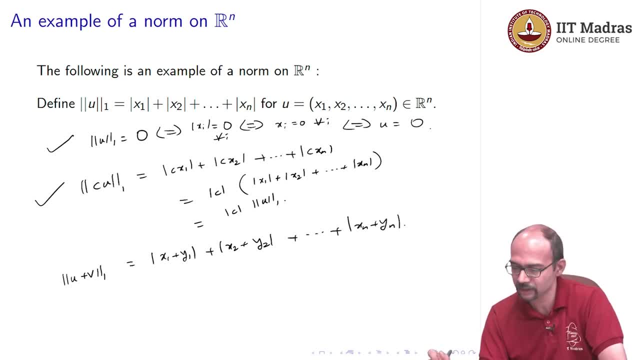 plus xn plus v. Well, let us write that down. That is x1 plus y1 plus x2 plus y2 plus xn plus v plus yn, where xi are the coordinates of u, yi are the coordinates of v. But we know that. 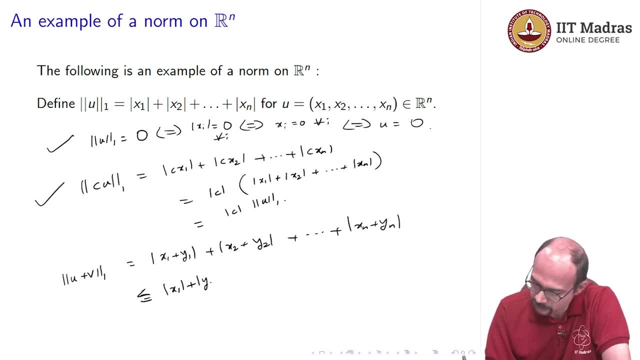 this is less than or equal to x1 plus y1,. this is less than or equal to x2 plus y2.. And then if you rearrange all these terms, you get that this is u1 plus v1.. So this tells you that it is a norm. So it is a fairly simple check that it is a norm. 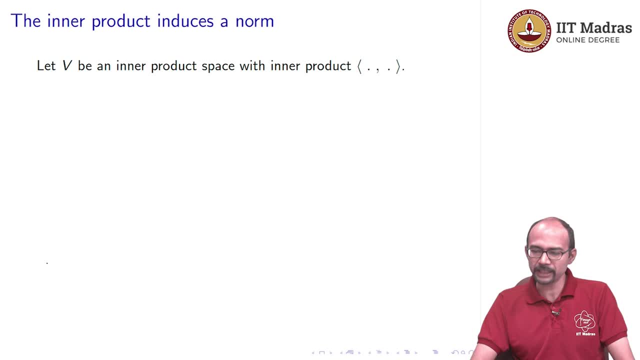 So, finally, let us explore the relation between the inner product and the norm. So suppose you have v, which is a inner product space, So it has an inner product which we have represented by these angle brackets. Let us define this function. So this function is norm of v is equal to square. 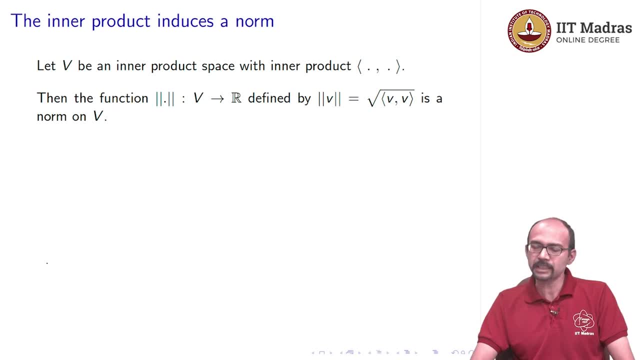 root of the inner product of v with its self, Then the claim is that this is the norm on v. Let us work this out. why this is the norm. So, first of all, norm of v is 0.. This happens exactly when the square root of the 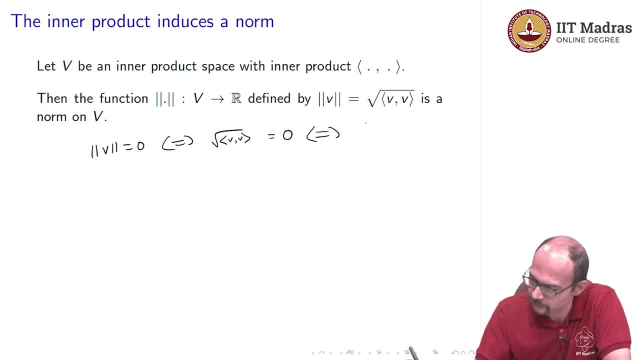 inner product of v with itself is 0, which happens precisely when the inner product itself is 0. But remember, it is an inner product. This happens precisely when v is 0. So I want to prove that this is always positive if 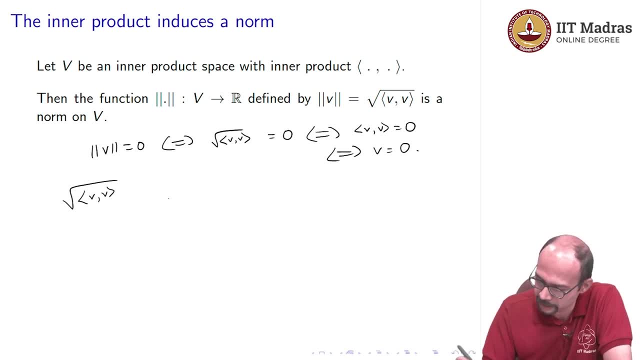 if v is non zero, but remember that v comma v is. so if d is not equal to 0, v comma v is greater than 0, that means square root of v comma v is strictly greater. we are always looking at the positive square root, which means norm of v is strictly greater than 0. So the 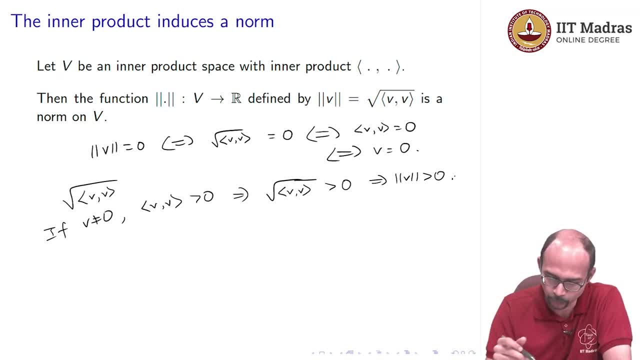 positive, non-negative and positive part is proved. that axiom is proved. So the other two axioms are the triangle, inequality. and if you multiply a scalar, what happens? Let us look at scalar. So for the scalar, so we have c times v. by definition, this is cv, comma, cv. 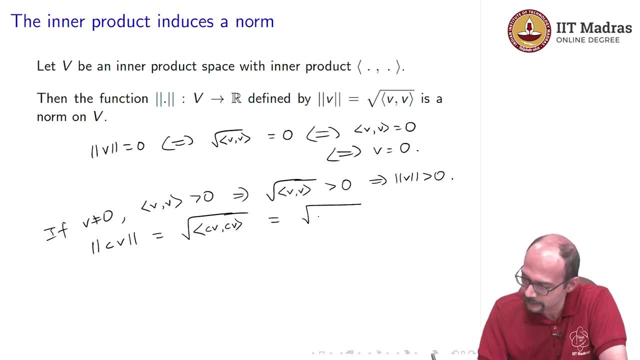 But, as we know, c comes out, so this is root of c, So it comes out of the first one and it comes out of the second one. So c times c. excuse me, this is norm of v, inner product of v, comma v. 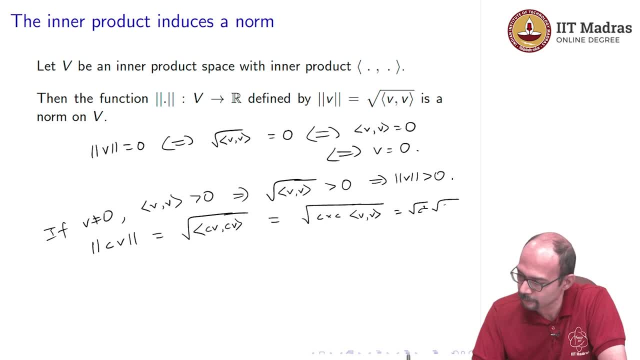 So this is root of c squared, root of v, comma v. The second part is exactly the norm of v And the first part is mod, of meaning the absolute value of c, because you are taking root of c squared. So if c is a negative number, after taking square root you always look at the 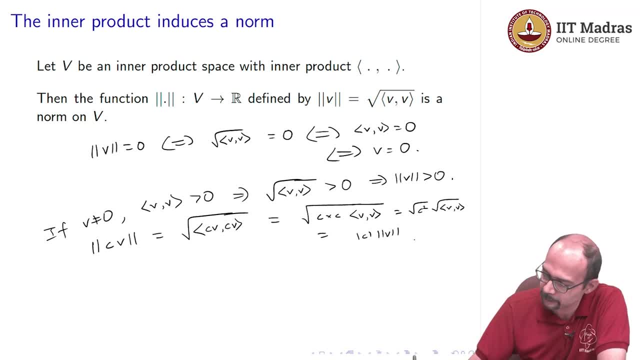 positive part, So it is the absolute value of c times norm of v. So this is another one of the axioms. And finally we have: if you have v plus w, by definition this is v plus w comma, v plus w square root, And this is so. you have four terms. You have v comma w plus w comma v. 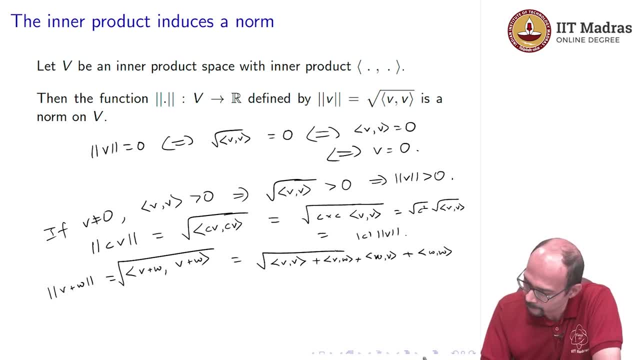 plus w, comma w, which, if you rewrite this, is v, comma v, And this is remember, it is a inner product, So it is. so we got the first thing by bilinearity, And then because it is symmetric.